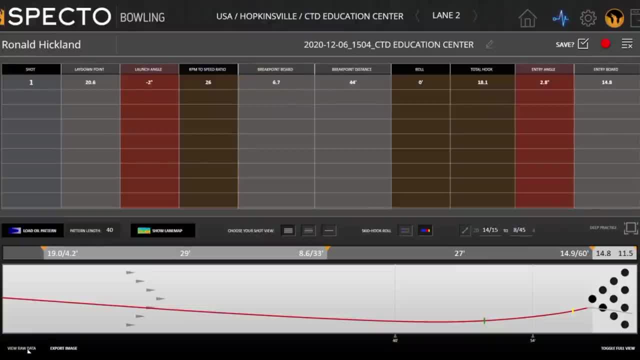 one of the cool things about Specto is we're going to be able to see the lay down point, the launch angle, and RPM to speed ratio is a way for us to verify that Dustin's throwing the shot. the same, We'll also look at the break point board. break point distance, the roll distance. 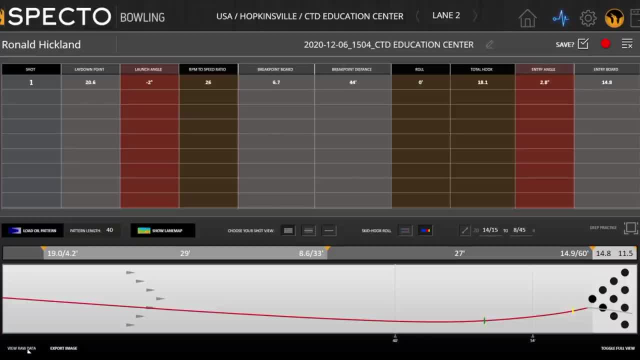 and the total hook is That kind of matters, right, That 18.1 total kind of matters a lot- Entry angle and the entry board. So now what we're going to do is we're going to throw the second ball, which is the pin down ball, which is 45 by five, by 75. And we're going to watch. 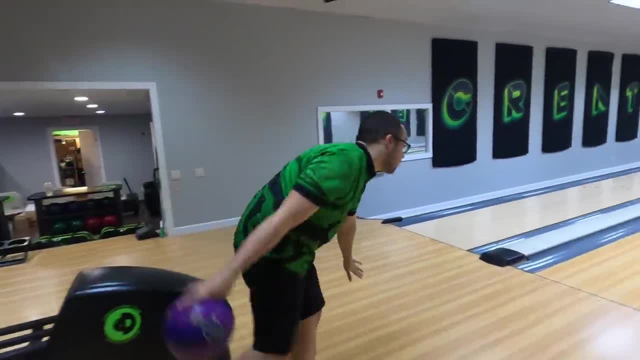 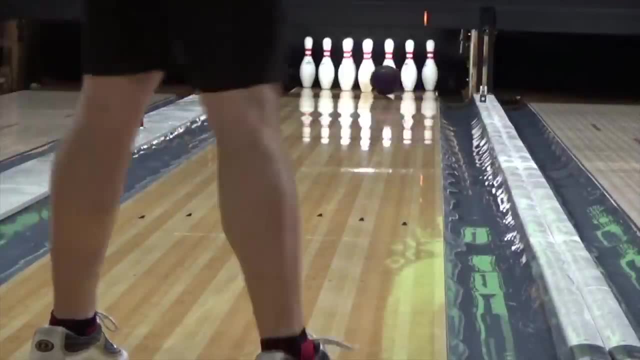 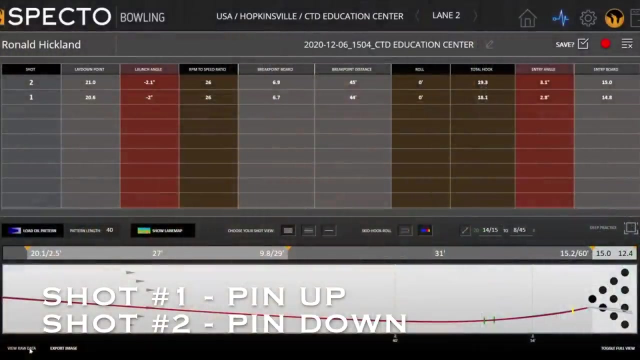 it go down to lane two. Got him a little strike right there. Now, look, this is awesome because we can get a look at the Specto data and really really compare these two bowling balls. You can see that second bowling ball was thrown less than four-tenths of an inch different at the lay down. 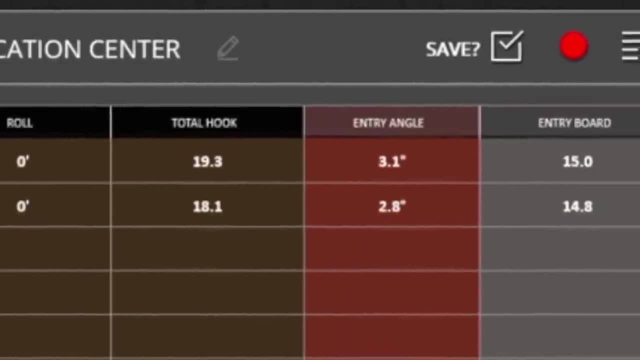 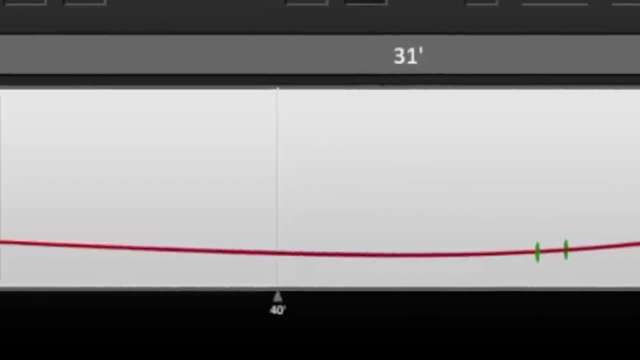 point. The launch angle is one-tenth of an inch. So basically these balls were thrown the exact same. So this is a very, very good comparison between pinup and pinned up. So going across the board, RPM to speed ratio is the same. The break point board was two-tenths. So I mean that's. 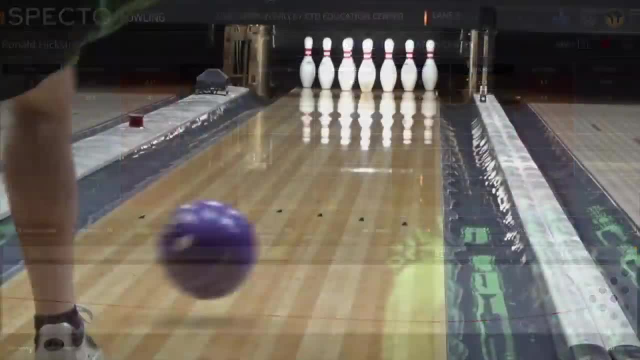 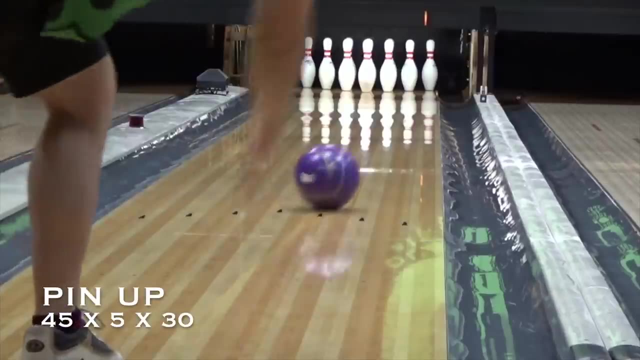 nothing. The break point distance was one-fifth of an inch, So we're going to take a look at the distance was one foot. the both balls with the ball got into a roll. the total hook was 19.3 for the pin down and 18.1 for the pit up. so a slight difference, right, a little more than a board. 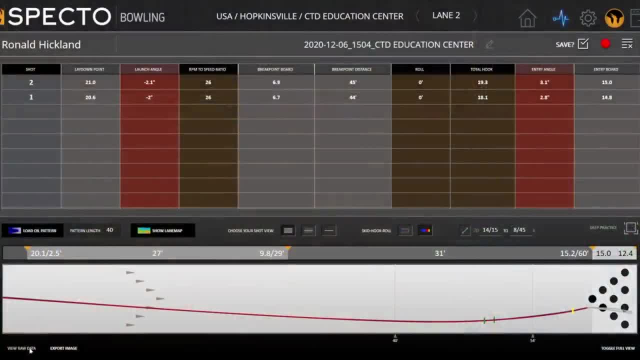 difference in total hook. the entry angle was also slightly more right, from 2.8 to 3.1, and the entry board was a little bit higher. so here's what's funny: when you're looking at this data on your screen, it doesn't look that different. right? that's because the truth is it's not that different. we're. 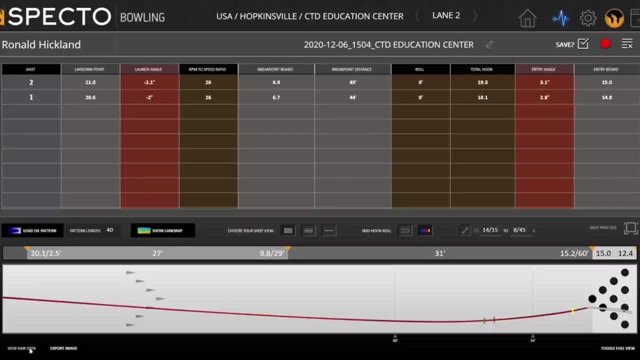 using a high quality, high caliber type of technology to even be able to see the difference between these two bowling balls. and obviously there isn't a whole lot of difference. now, if we take a look at some of the flare potential of the bowling ball, the flare on the pin down ball is a 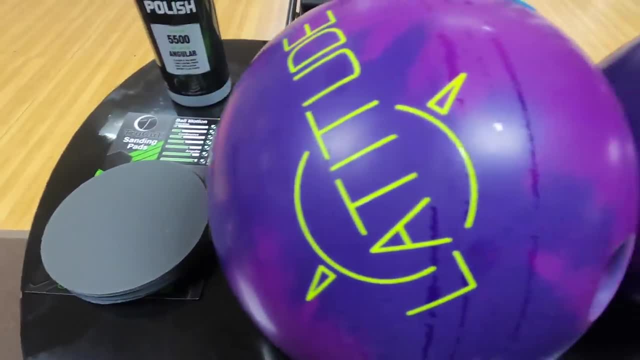 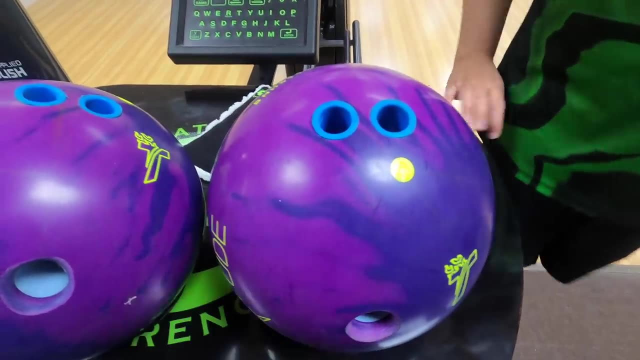 little bit different, as you can kind of see there, than the pin up ball. so there's a little bit of difference in the way the ball flares. one of the big concerns people run into a lot of times with pin down balls is they worry about it clipping the hole, and the reason being is because as you move,